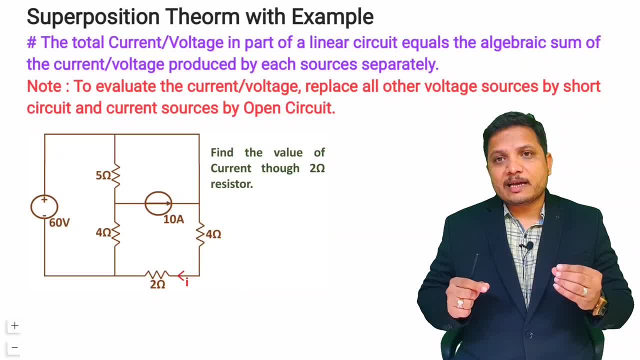 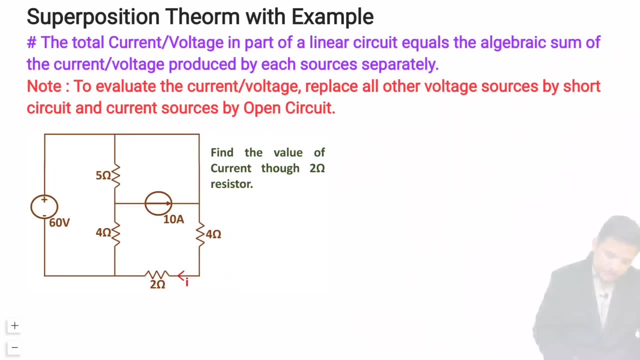 explain what is the basic theoretical part which is there with superposition theorem. So I thought I should explain what is that theorem which is being used in electrical network. So let us see first what is the basic theorem which is there with superposition theorem. So, my dear students, here, superposition theorem is used to identify voltage or current. 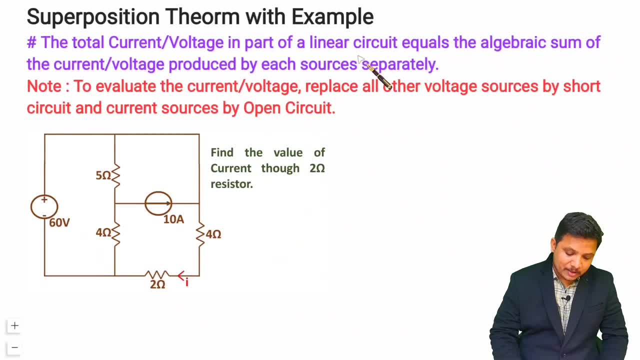 through any linear element right, And the total current or voltage in a part of linear circuit is equals to the algebraic sum of current voltage produced by each sources separately. So for example, here you see, here we are having circuit in that we are having 60. 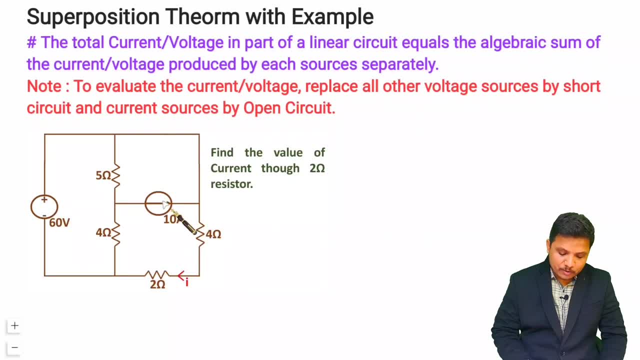 voltage battery over here and 10 ampere current source over here, right And we are delivered to find current passing through 2 ohm resistor. So when you want to find current passing through this 2 ohm resistor, then you will have to find current passing through 2 ohm resistor because of 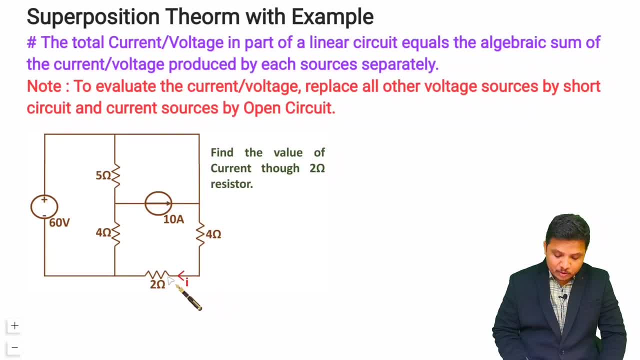 60 voltage battery as well as current passing through this 2 ohm resistor. because of 10 ampere current source, An algebraic sum of both will be total: current passing through this 2 ohm resistor. That is what the basic definition which is represented over here. Now, here one thing that 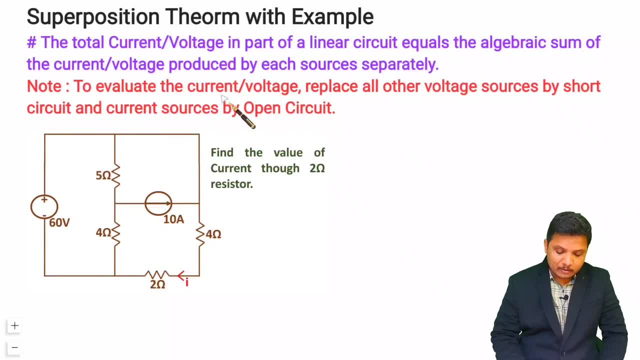 you need to note down when you evaluate current or voltage. all you need to do is you will have to replace the current passing through this 2 ohm resistor. So you will have to replace the current passing through this 2 ohm resistor. So you will have to replace all the voltage sources by 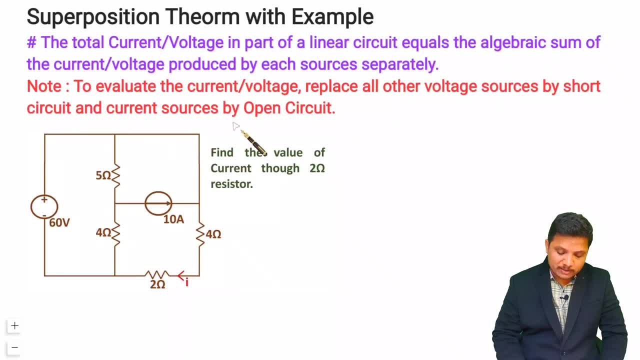 short circuit and all the current sources by open circuit. So I will show you how to provide short circuit instead of voltage source and how to provide open circuit instead of current source. So let us try to understand that by this practical example. So if you observe in this question, 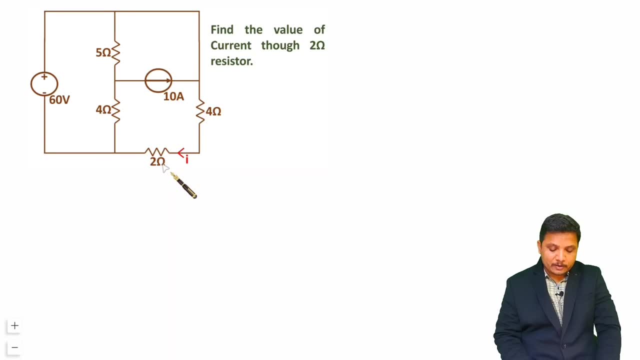 we are delivered, to find current passing through 2 ohm resistor. So, my dear students, what we will do is, first I will be identifying current passing through 2 ohm resistor because of 60 voltage battery. So let me redraw this circuit first. Now I have redrawn the circuit right And now. 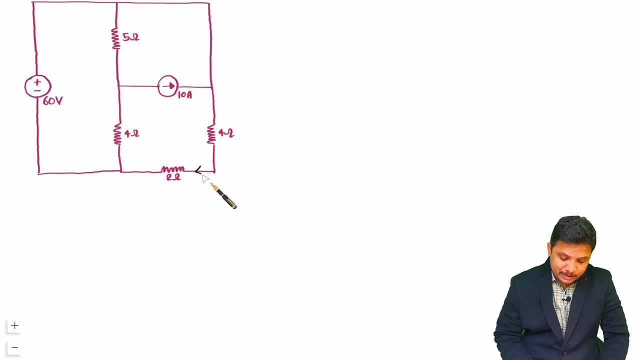 what I will do is I will calculate current passing through 2 ohm resistor because of 60 voltage battery, and let us say that is I1, right? So see, because of 60 voltage, we are delivered to find right. So other voltage sources should be short circuited and current sources should be open. 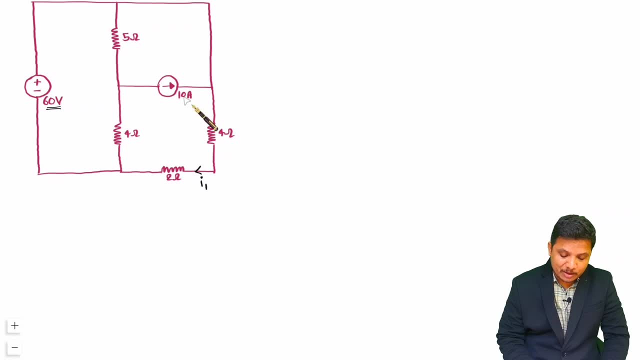 circuited. So see this current source of 10 ampere that should be open circuited. So let me remove this. Now we are just delivered to find what is the value of I1 because of this 60 voltage source. 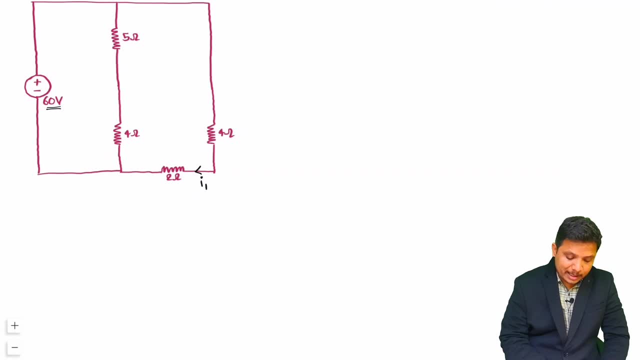 So you see this 60 voltage that is applied across this 2 terminal right. So what is current I1? Current I is voltage divided by resistance right As in between these 2 terminal voltage is 60, right And resistance of this wing, that is series of 2 and 4.. So 2 plus 4.. So that is 60 divided. 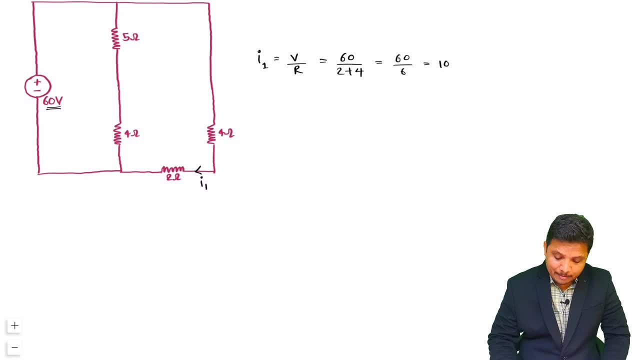 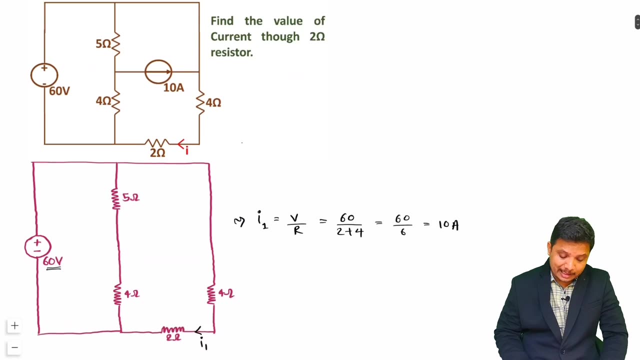 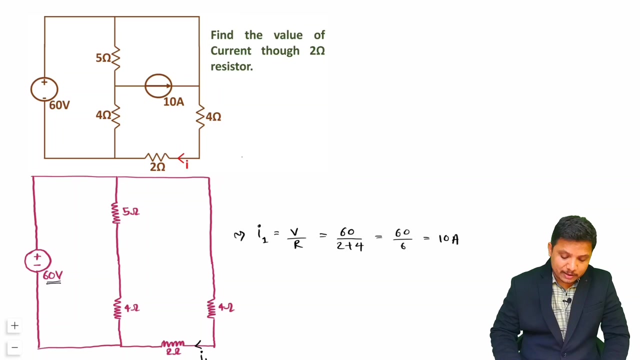 by 6.. So I can say: this is 10 ampere. right Now, my dear students, what I will do is I will be passing through 2 ohm resistor because of 10 ampere current source. So what I will do is now: 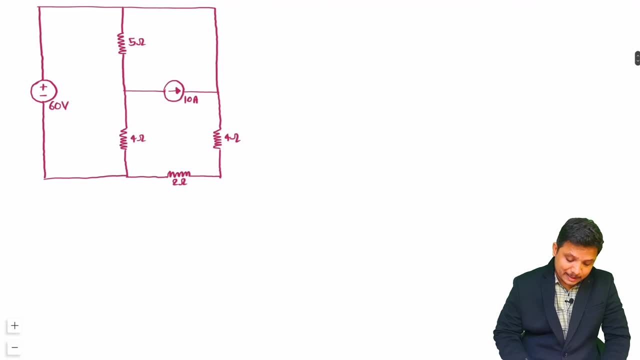 I will redraw this circuit first. Now let us say current passing through 2 ohm resistor, that is, I2, and now what I will do is I will be considering 10 ampere current source, So this voltage source that should be short circuited right. So what I will be doing is I will be removing this voltage. 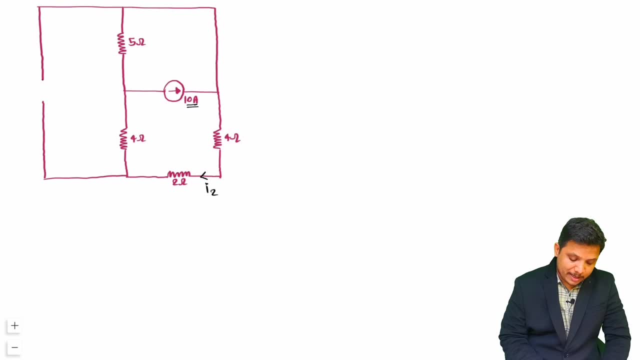 source now and instead of that I need to provide 10 ampere current source. So this voltage source short circuit right Now, when you have this 10 ampere current source, how to find I2?? So when you see this circuit initially, at that time you will be observing this connection is bit awkward. 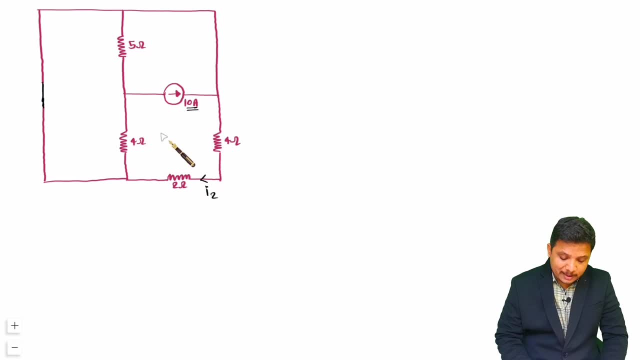 So all you can do is you can redraw this circuit right. Why? the reason is: you see, here there is a short, Here there is a short. So what is getting shorted? That is bit difficult to identify directly by viewing this circuit. 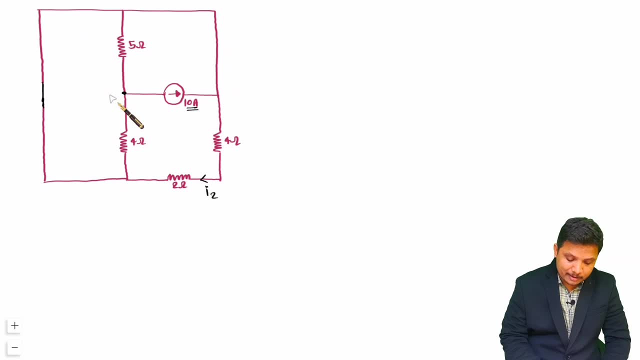 So what I will be doing is: let us say this is point A and let us say this is point B. So what I will do is I will redraw this. So here I am placing point A and here I am placing point B. 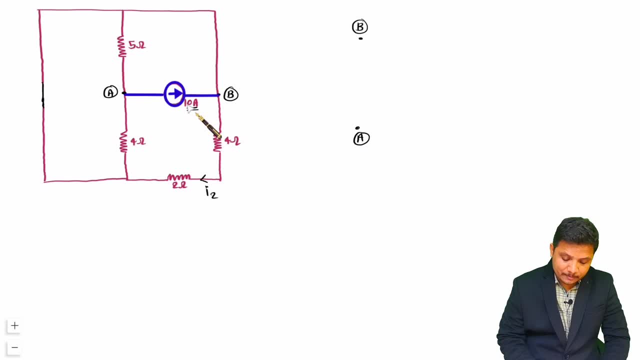 So see A to B. current source is there with 10 ampere, So let me draw it over here. Now let us try to understand how this 5 ohm resistor is connected. So see this B terminal that is shorted over here. So this is B terminal, right? So you? 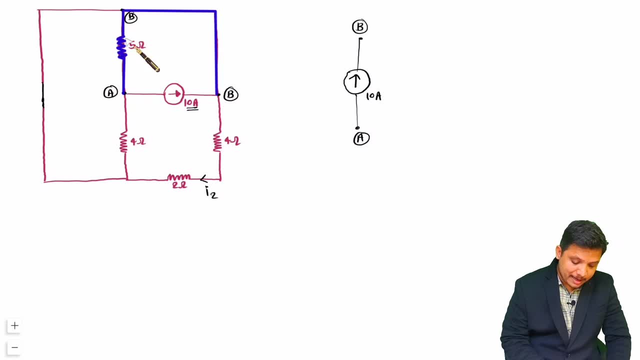 see this 5 ohm that is there in between A and B. So let us connect this 5 ohm in between A and B right Now. if you observe, see this, B is shorted over here, So this is also terminal. 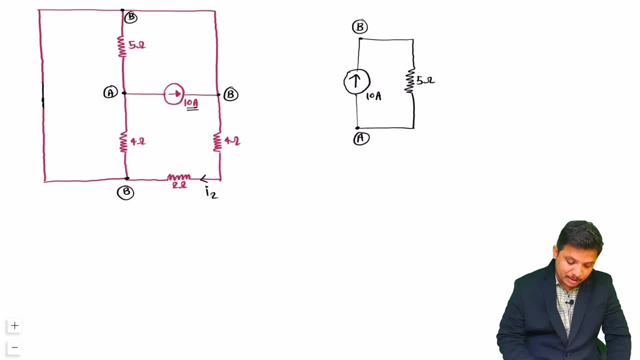 B right. So if you observe, in between B terminal, this wing is connected right, Which is of 2 ohm and 4 ohm in series. So you see how connection is there From B to B resistance. 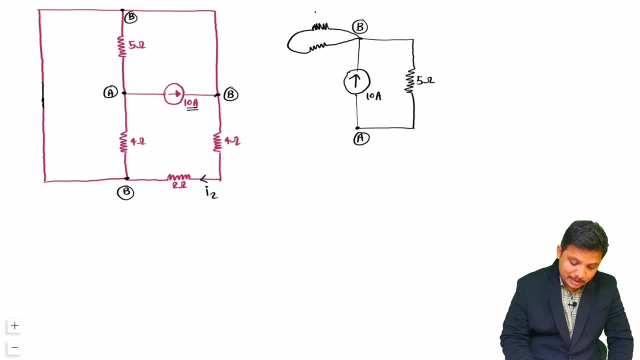 are connected like this right: One resistor is of 4 ohm and one resistor is there of 2 ohm Right And right- See now I2. that is happening like this right. So that is how B to B connection is there. 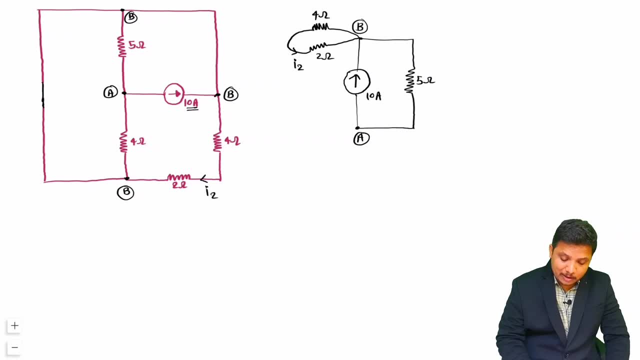 So now question is: what is I2?? Now you see across this: two resistors potential is same, which is B. So if potential difference is 0, how much current will pass through this wing? It will be 0, obviously, right, As here potential is fixed. So potential difference. 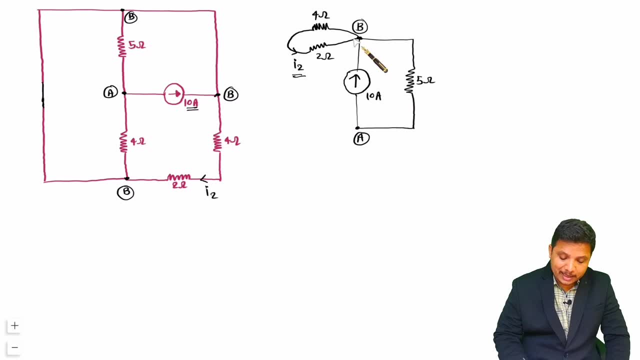 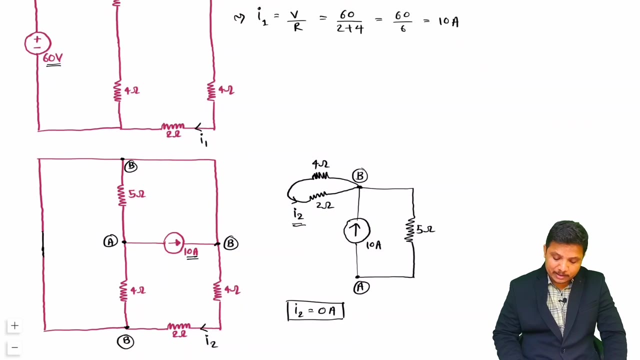 across this two resistor is 0. So I can say I2 over here that will be 0 ampere, right? So as per superposition theorem, total current, that is I1, which is 10 ampere, plus I2, which is 0 ampere, So total I that.